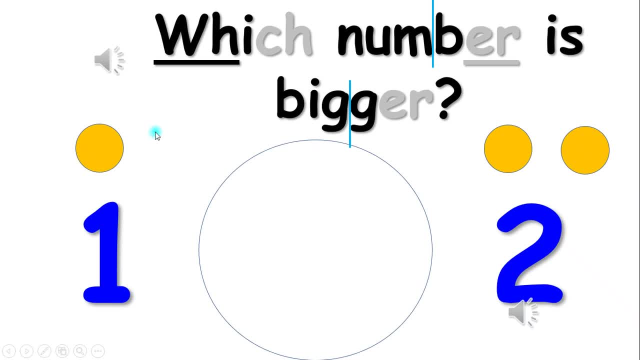 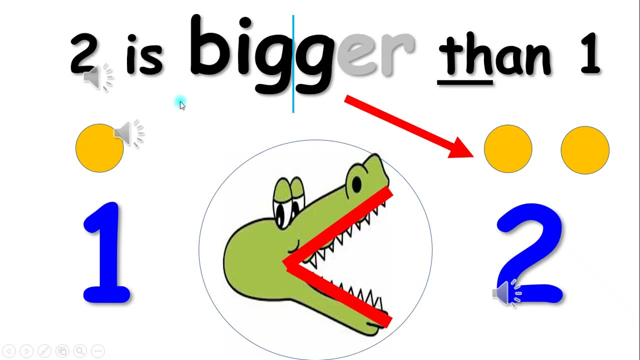 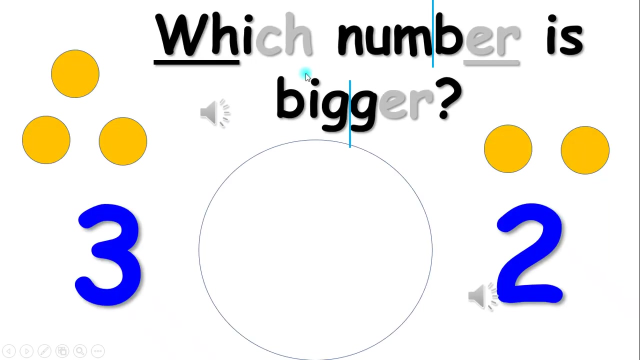 Which number is bigger, one or two? Very good, You are right. Two is bigger than one because two has more dots than one. Notice how the alligator's mouth is open to the bigger number. The alligator opens his mouth to the bigger number. 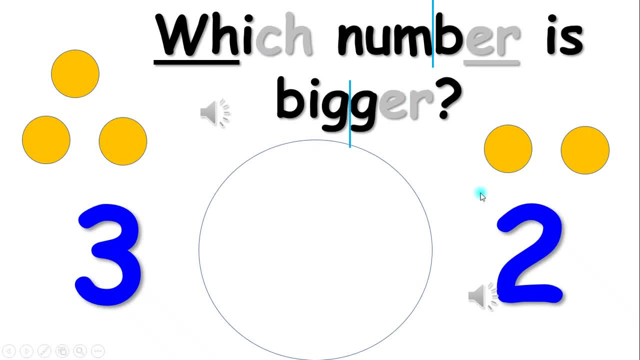 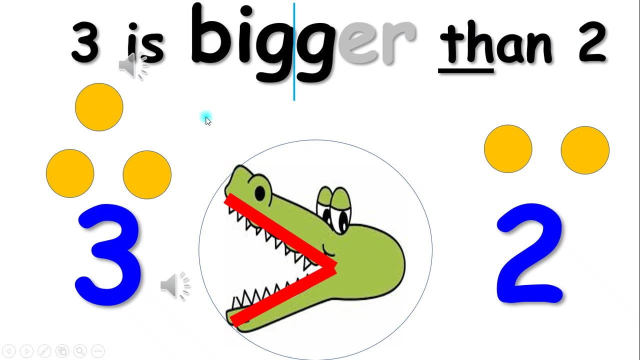 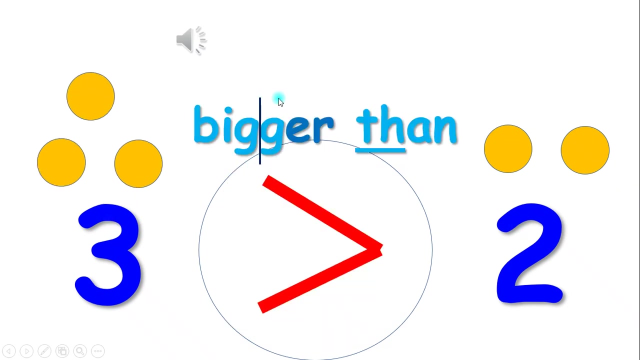 Which number is bigger? Is it three or two? Good job, Three is bigger than two. As you can see here, the alligator always opens his mouth to the bigger number, which is three. Three is bigger than two. Instead of saying bigger than, you say greater than. 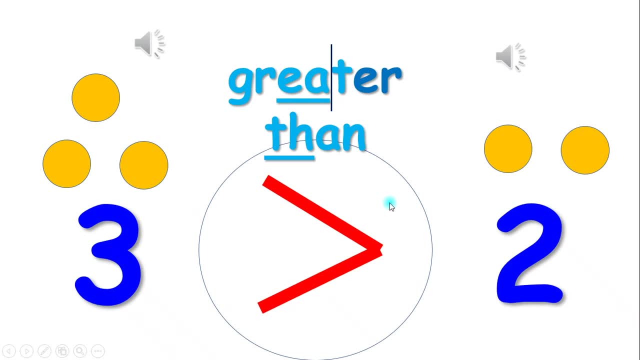 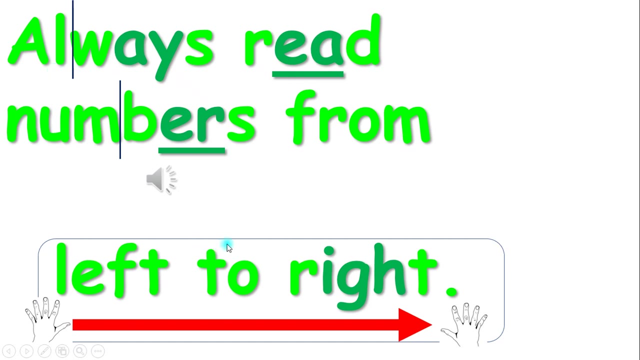 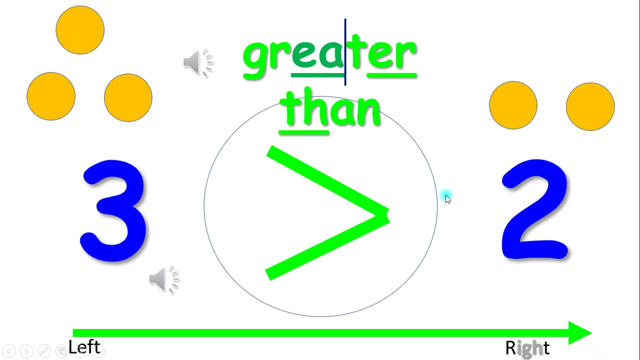 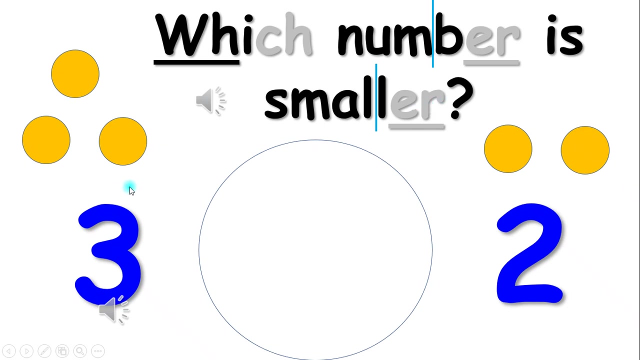 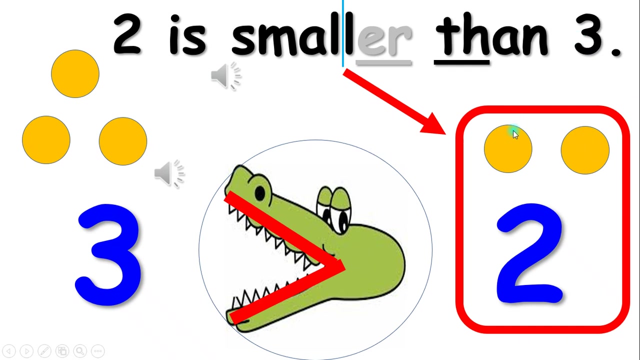 Three is greater than two. Always read numbers from left to right. Three is greater than two. Which number is smaller? Two is smaller than three. Very good, Two is smaller than three. Notice how the alligator doesn't open his mouth to the smaller number. 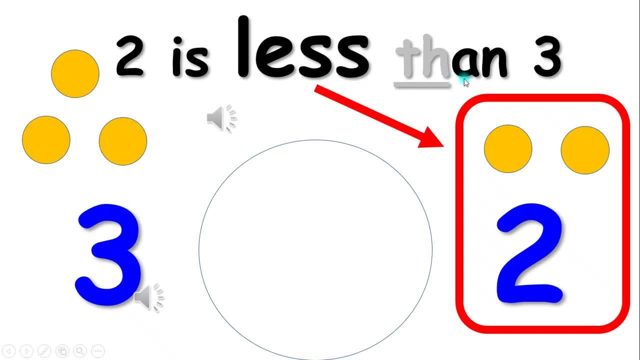 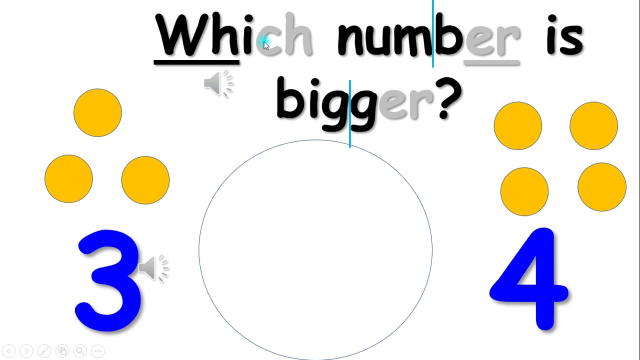 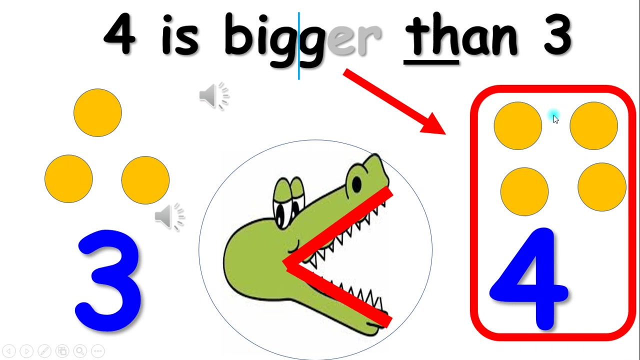 Instead of saying smaller than you can also say: less than Two is less than three. Which number is bigger? Is it three or four? You are right, Four is bigger than three, because four has more dots than three And the alligator always opens his mouth to the bigger number. 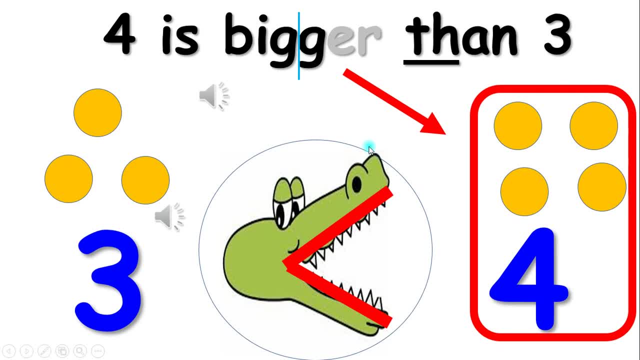 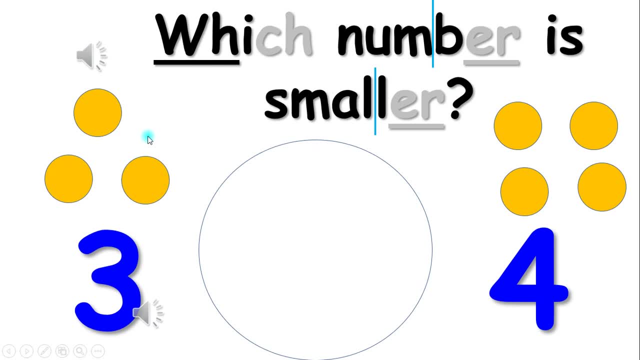 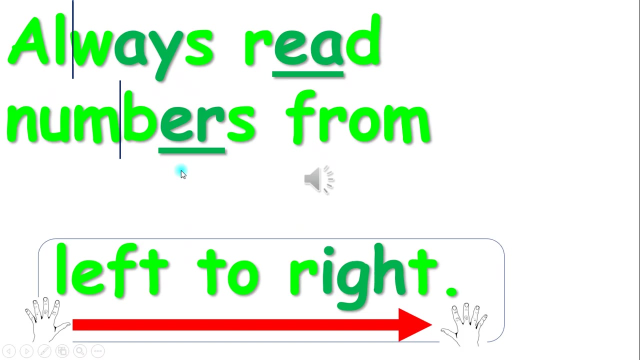 The alligator opens his mouth to the smaller number. Which number is smaller? Three is smaller than four. Good job. Three is smaller than four. The alligator opens his mouth to the smaller number. Three is less than three. Three is less than four. 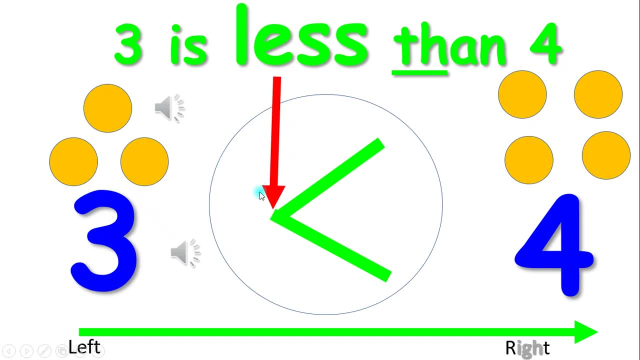 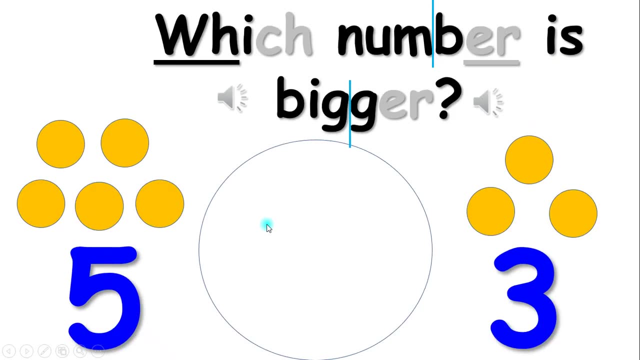 The back part of this open mouth means less or smaller. Three is less than Mr Bigger. The pervert opens his mouth to the smaller number. The pervert opens his mouth to the larger number. Three is less than four. The back part of this open mouth means less or smaller. 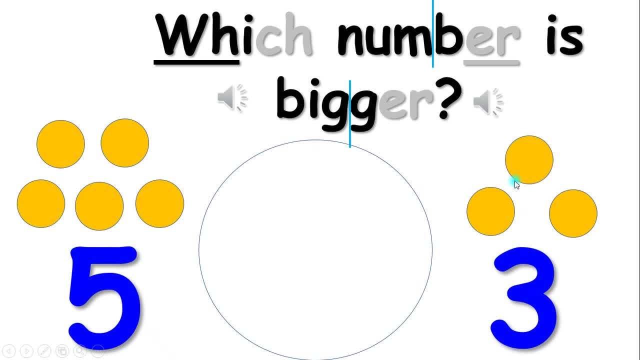 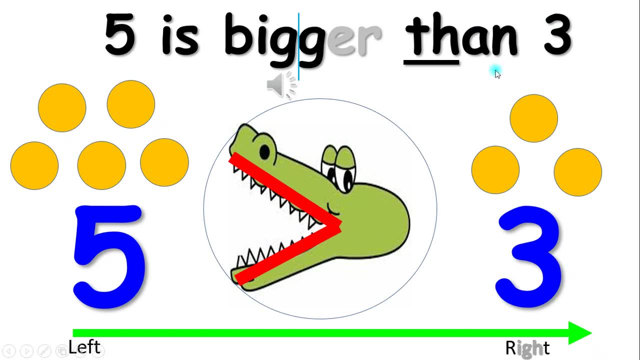 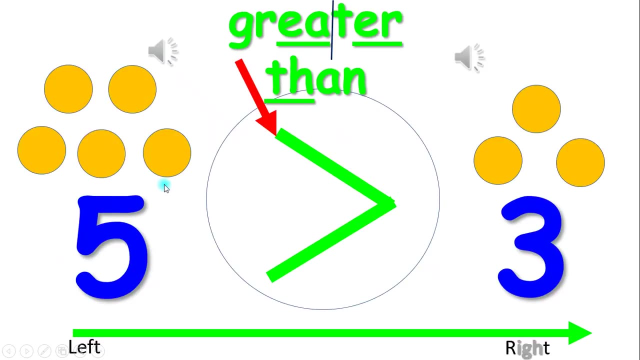 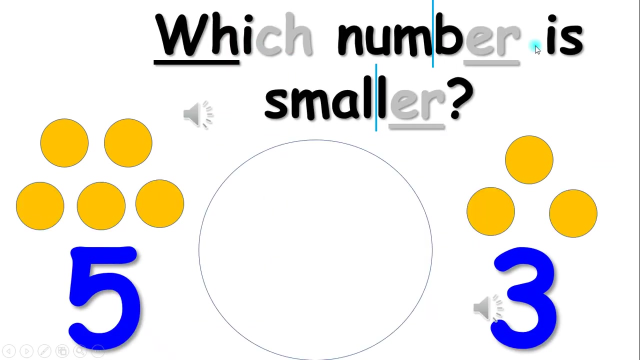 Which number is bigger? Is it five or three? Good job, Five is bigger than three. Five is greater than three. The open mouth means greater. Five is greater than three. The open mouth means greater. Which number is smaller? Is it five or three? 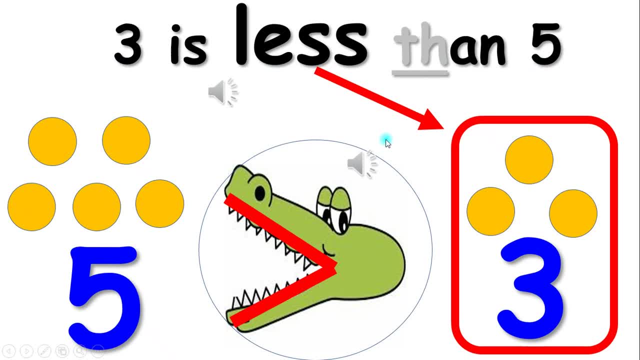 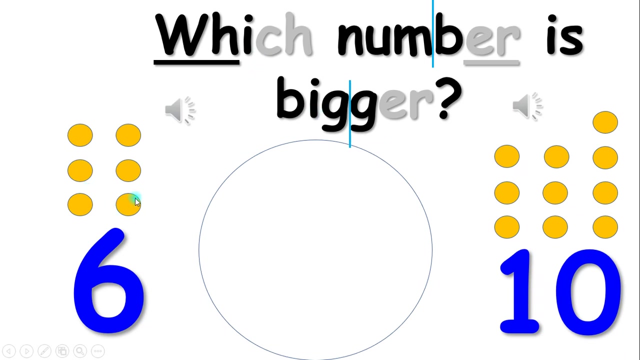 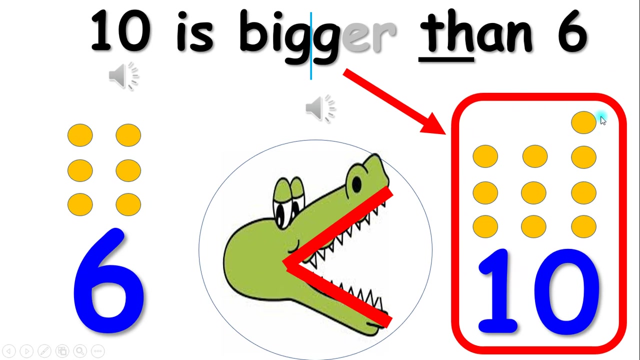 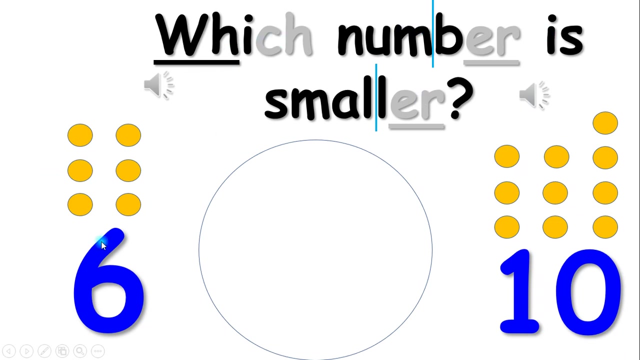 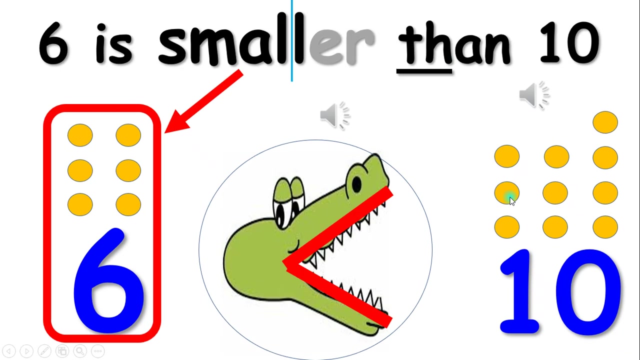 Three is less than five because three has fewer digits And the alligator does not open his mouth to the smaller number. Which number is bigger? Six or ten? Ten is bigger than six. Which number is smaller? Six is smaller than ten. 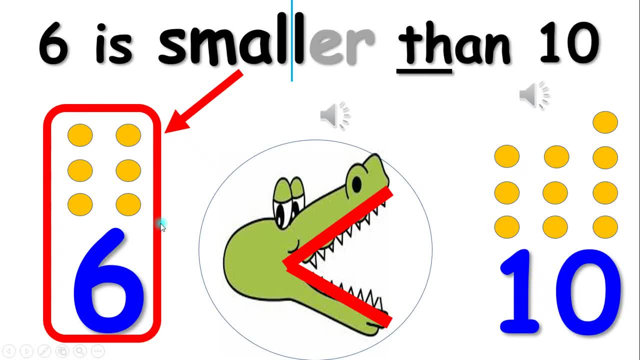 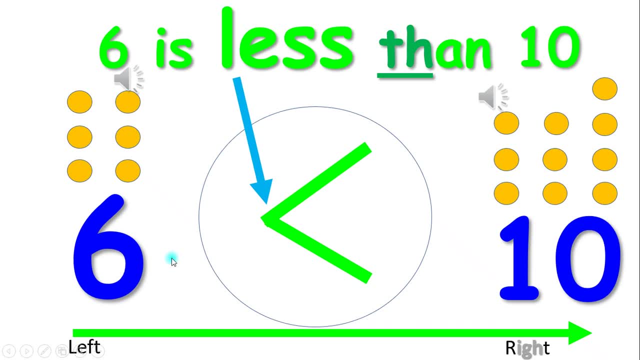 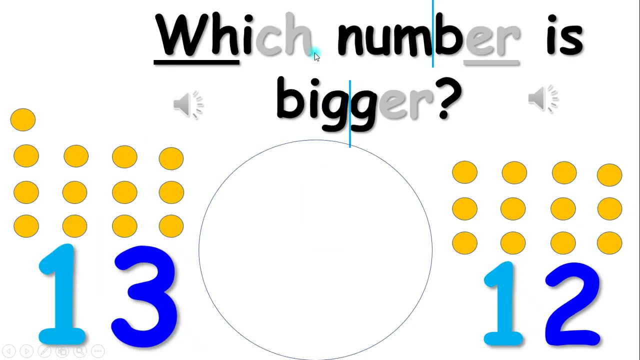 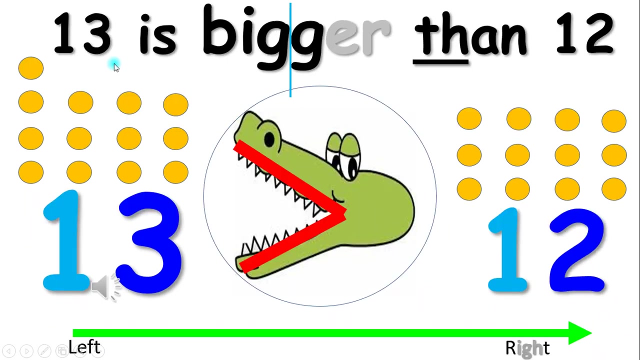 The answer is four. Six is less than ten. Ten is bigger than ten. Which number is smaller than five? Six is less than ten. Which number is bigger? Is it 13 or 12?? 13 is bigger than 12.. 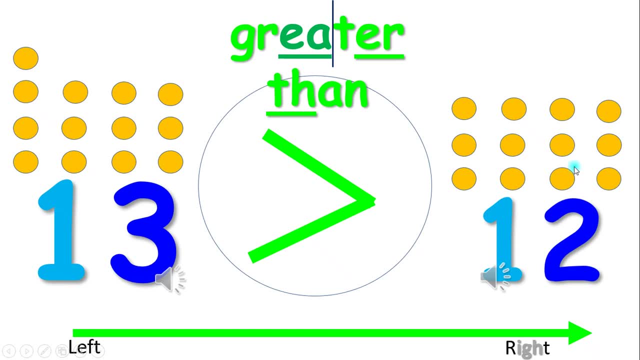 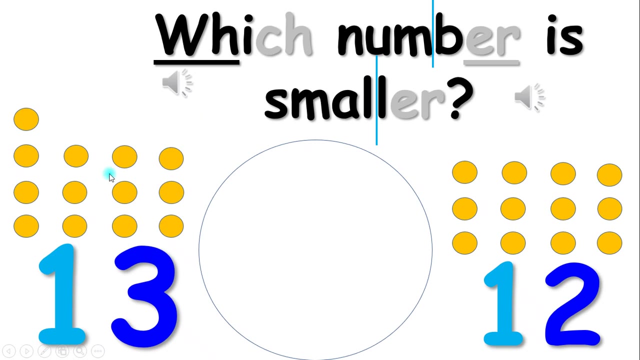 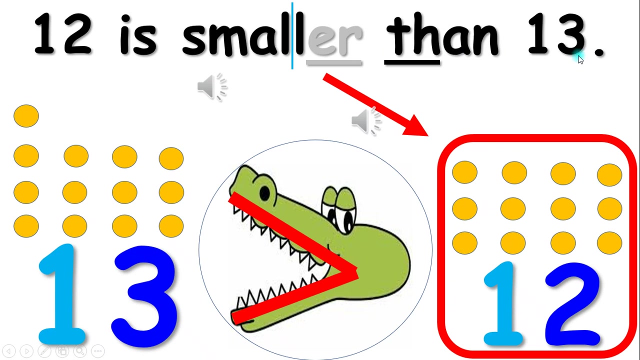 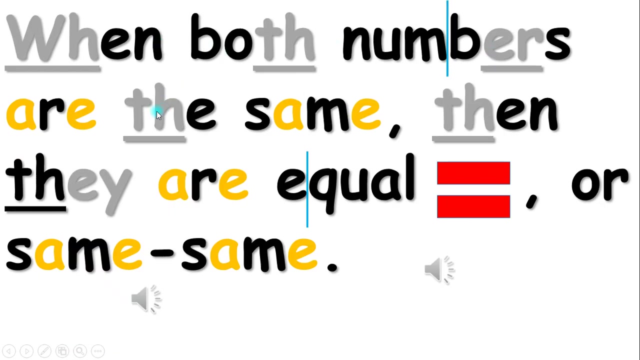 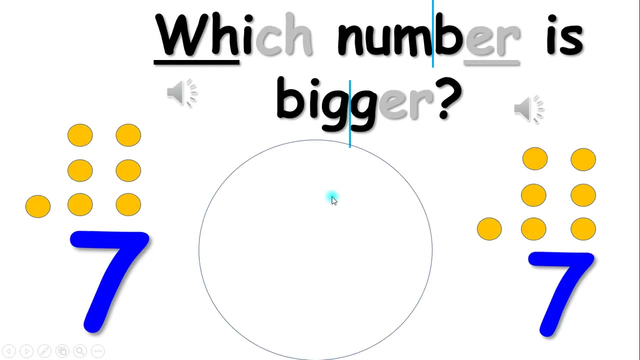 13 is greater than 12.. 13 is greater than 12.. Which number is smaller? 12 is smaller than 13.. When both numbers are the same, then they are equal or same-same. Which number is bigger? Is it 17 or 12?? 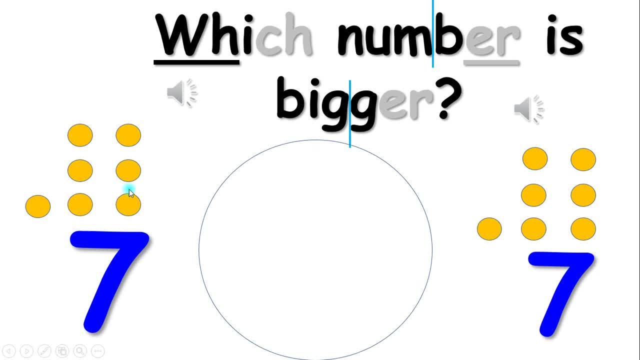 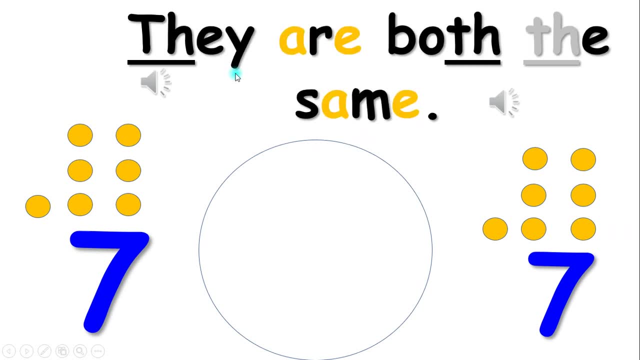 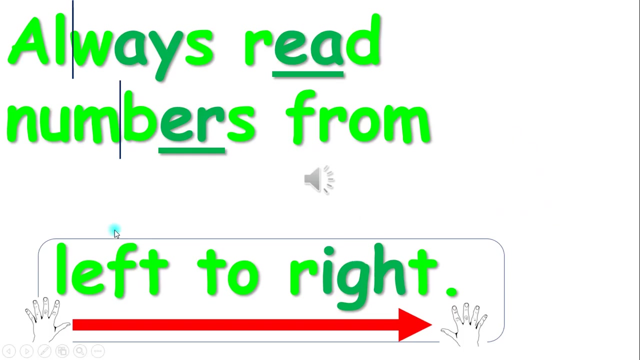 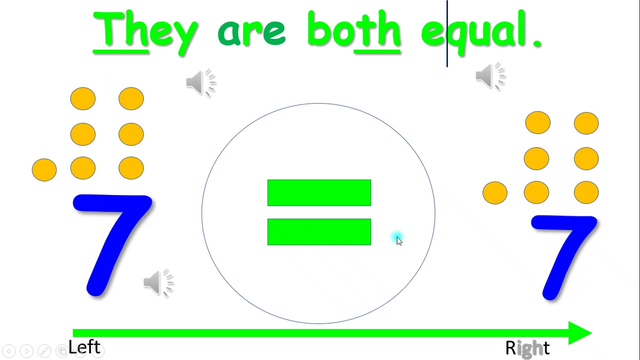 Is it 7 or 7?? Is it 7 or 7?? Is it 7 or 7?? They are both the same. When both numbers are the same, such as 7 and 7, they are both equal to each other. 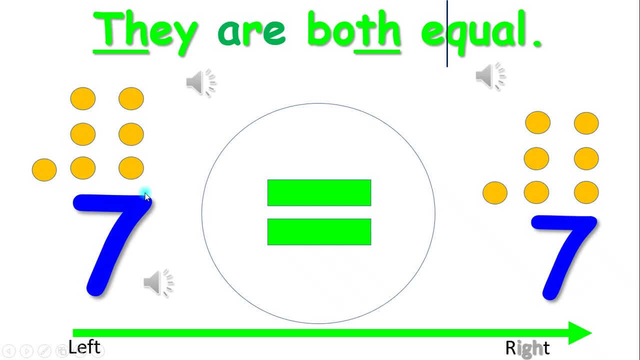 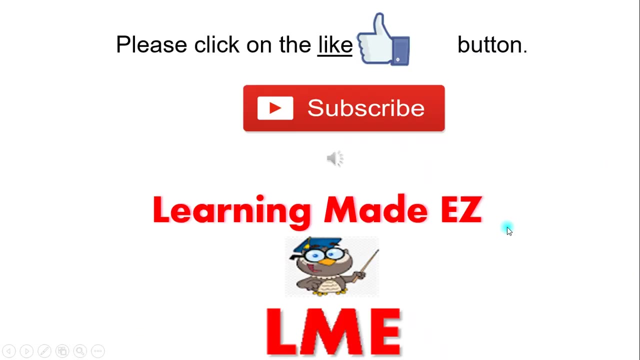 When both numbers are the same, such as 7 and 7, they are both equal to each other. You read it as 7 equals 7.. You read it as 7 equals 7.. What number is bigger, 5 or 9?? 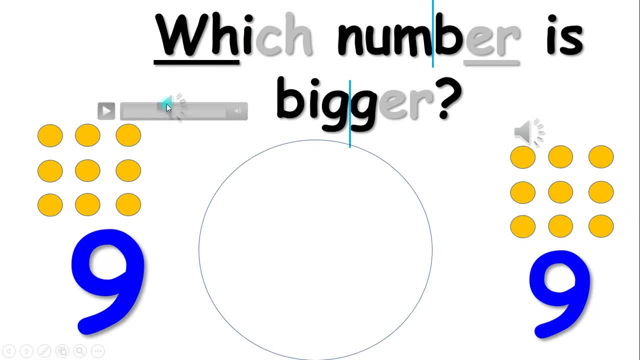 5 is 2 and 7 is 3.. Which number is bigger? Is it 9 or 9?? 9 is higher than 7.. 9 is lower than 7.. 8 is lower than 7.. When both numbers are the same, such as 3 and 7, they are equal to each other. 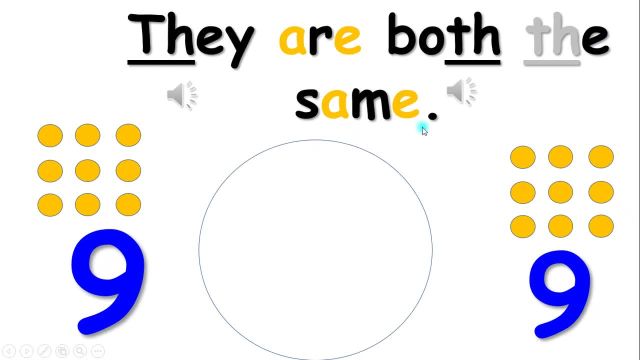 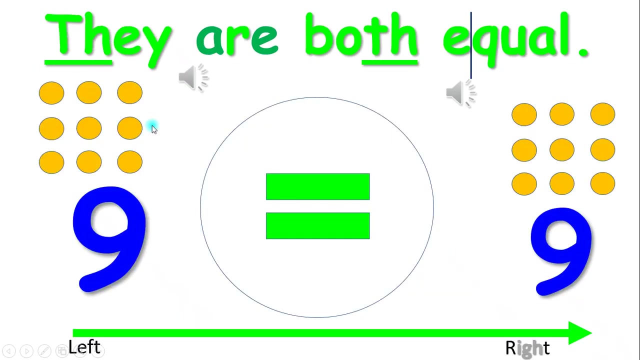 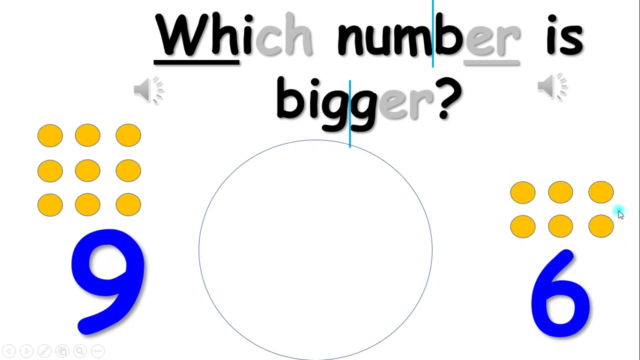 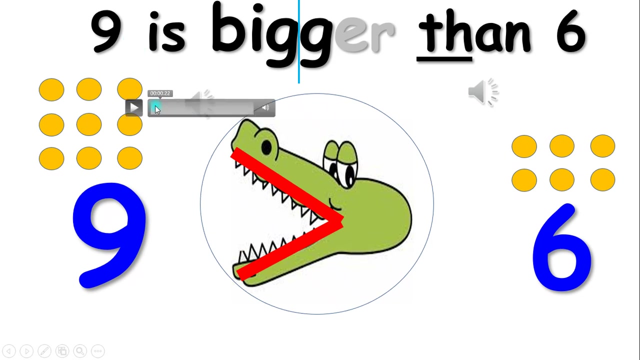 When both numbers are the same, such as 7 and 7, they are equal to each other. They are both equal. You read it as: nine equals nine. Which number is bigger? Is it nine or six? Nine is bigger than six. 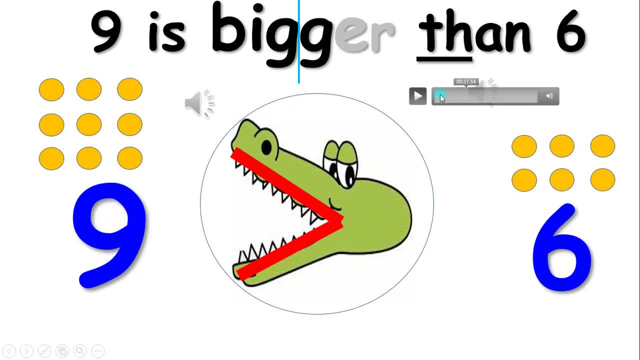 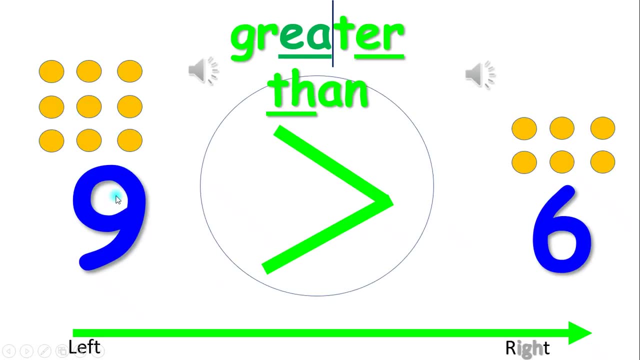 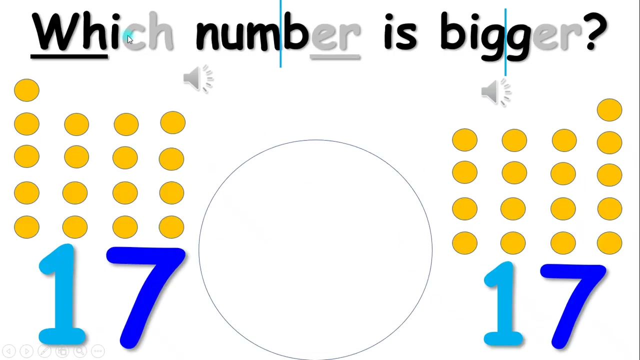 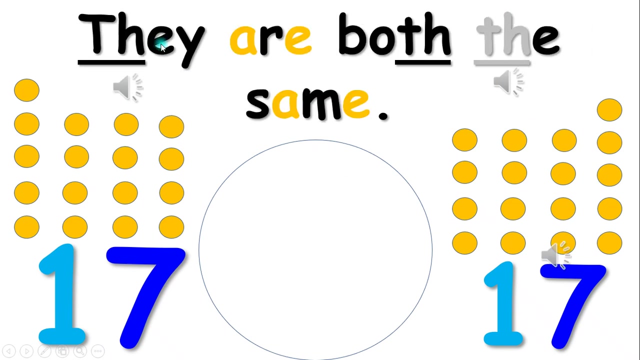 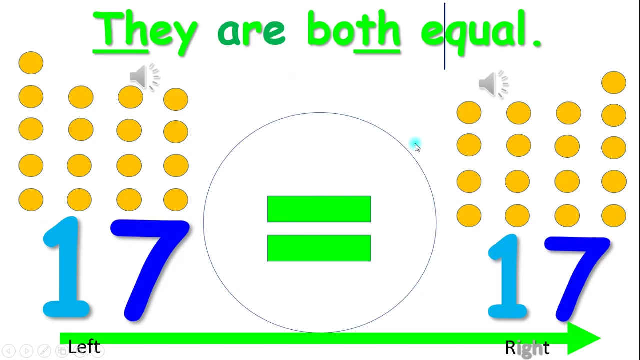 Nine is bigger than six. You read this as nine is greater than six. Which number is bigger? Is it seventeen or seventeen? You are right, They are both equal, the same. Both numbers have the same or equal amount of dots: Seventeens and seventeen, They are both equal. You read it as: 17 equals 17.. 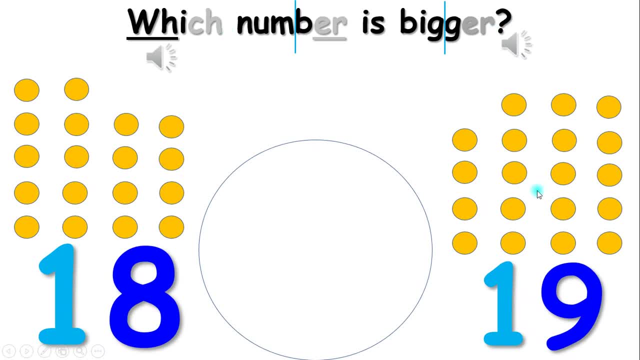 Which number is bigger? Is it 18 or 19?? In order to decide which number is bigger, you can count which number has more dots or use the number line to help you. Numbers going to the left on the number line become smaller, and numbers going to the right on the number line. 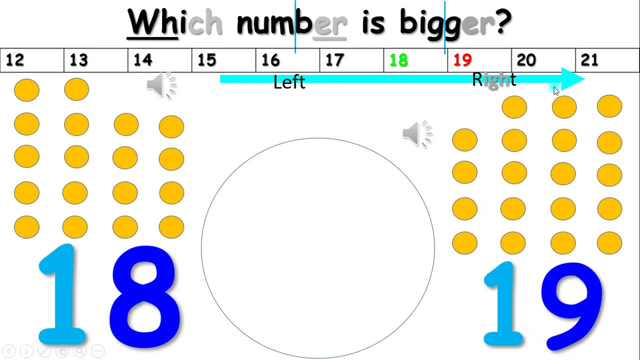 become smaller. So look at 18 and 19.. 18 is going towards the left and 19 is going towards the right. You did it, You figured it out. You figured out which number is bigger. 19 is bigger than 18 because 19 is going. 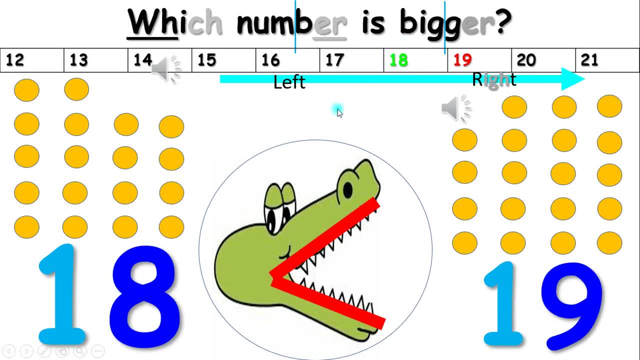 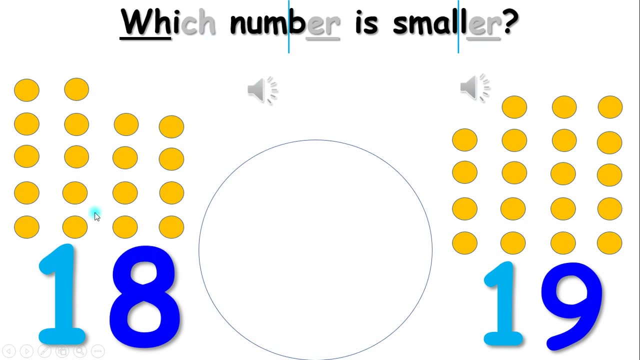 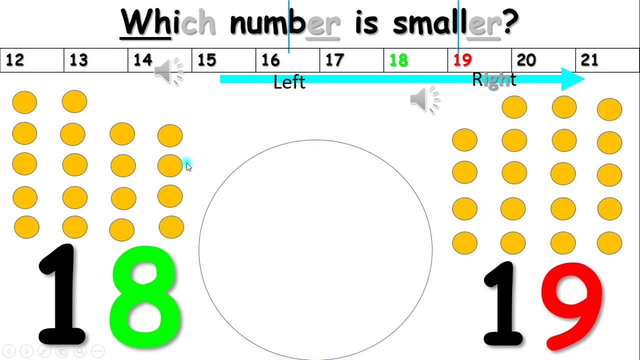 toward the right and 18 is going towards the left. Which number is smaller, 18 or 19?, 19 or 19.. Remember, You can use the number line to help you. Numbers going to the right are getting bigger and numbers on the left are getting smaller. So 19 is on the. 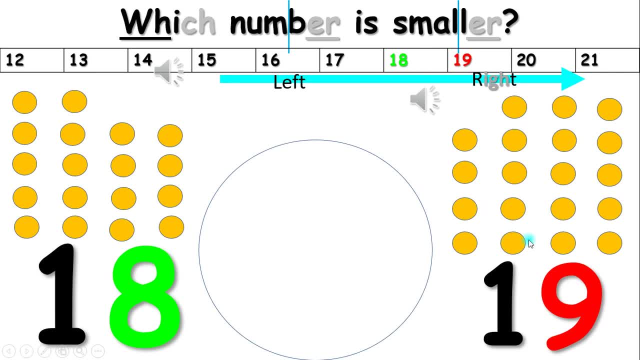 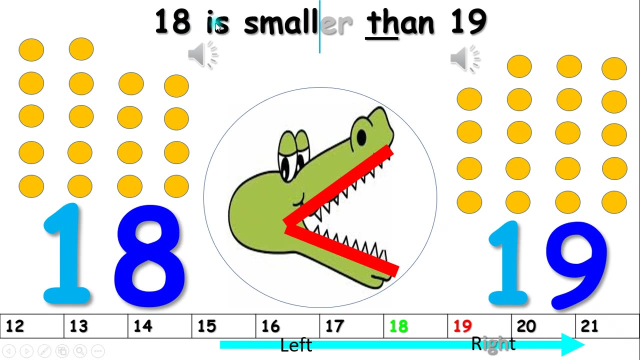 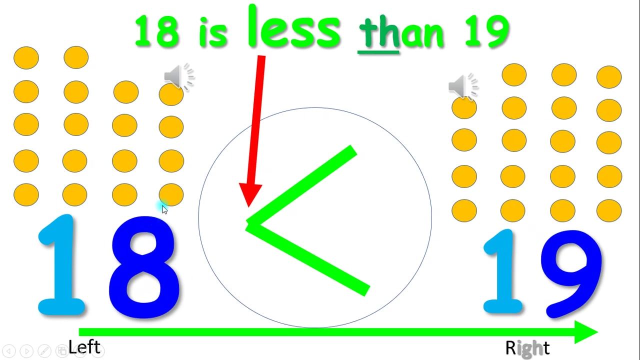 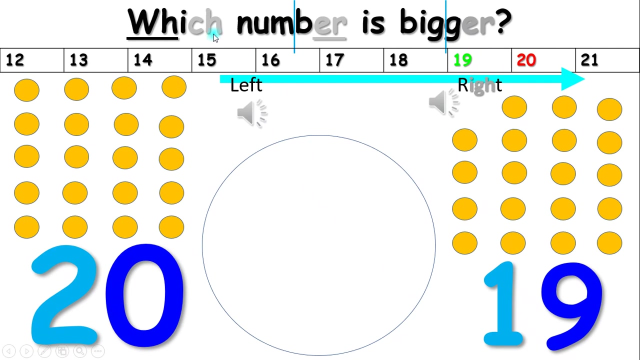 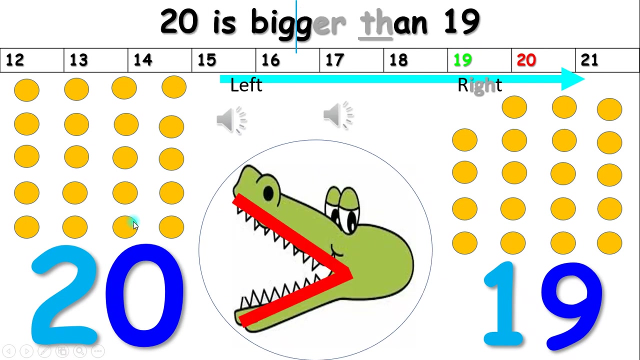 right and 18 is on the left. Good job, You figured out that 18 is smaller than 19.. 18 is less than 19.. The back part of this open mouth means less than or fewer than. Which number is bigger, 20 or 19?? 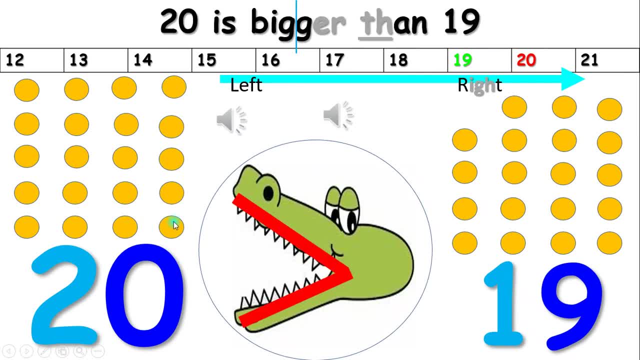 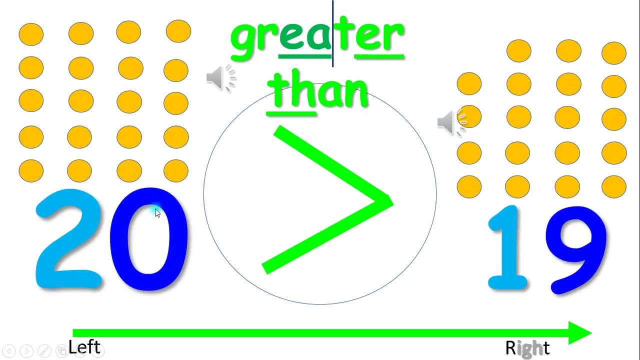 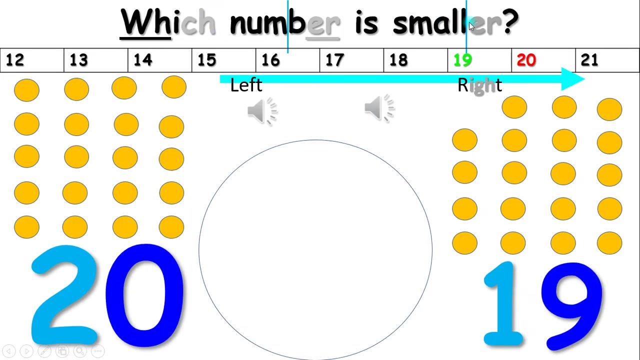 Good job. You figured out that 20 is bigger than 19.. You can read it as: 20 is greater than 19.. You can read it as: 20 is greater than 19.. Can you figure out which number is smaller, 20 or 19??